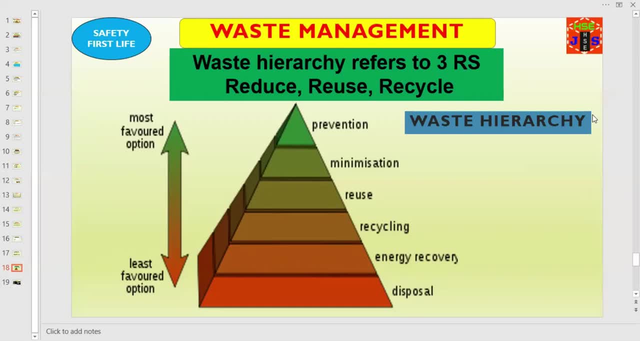 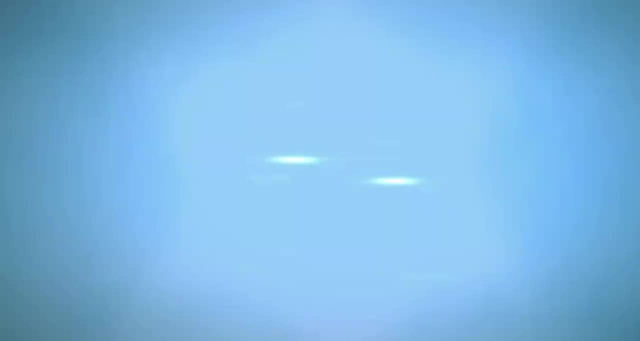 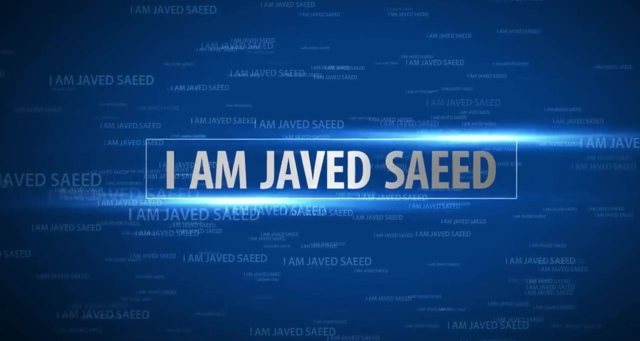 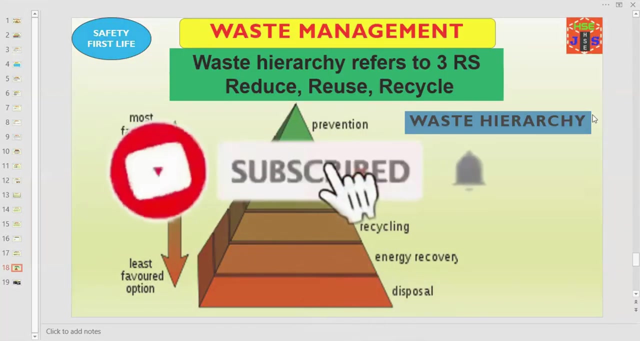 If the waste have this much consequences, it's important to understand how to control and manage waste wisely. For that purpose, you have to understand hierarchy of waste management. Hierarchy of waste refers to three R's: reduce, reuse and recycle Waste management. 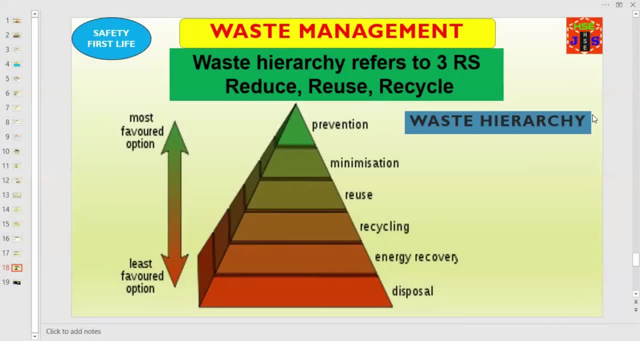 hierarchy starts from prevention. It is the most favored and number one option. The second favored option is minimization, Third, reuse, Fourth, recycling, Fifth, energy recovery. And the last sixth and the least favored option, disposal In the upcoming 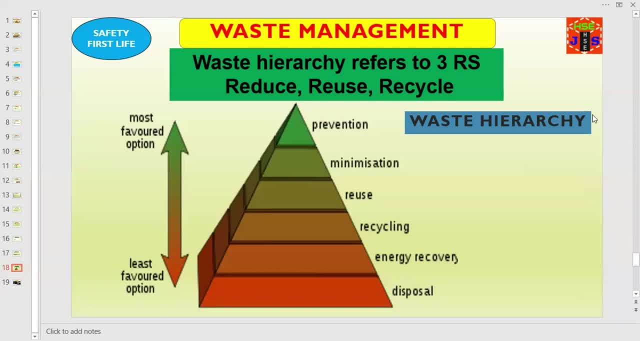 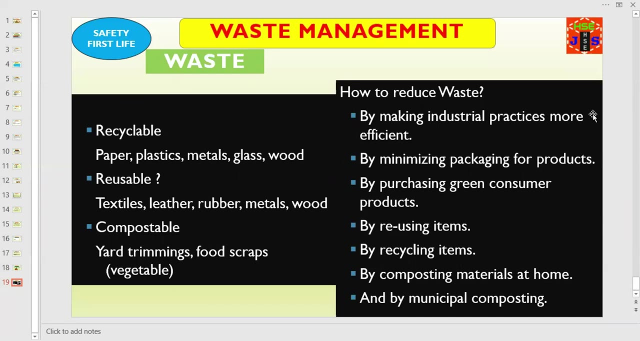 training session I'll tell you what are the different ways of waste disposal, how we can dispose of waste efficiently, safely And wisely. As I told you, the number one option is waste prevention, But practically it is not possible in all cases, So the second most favored option is to minimize or reduce. 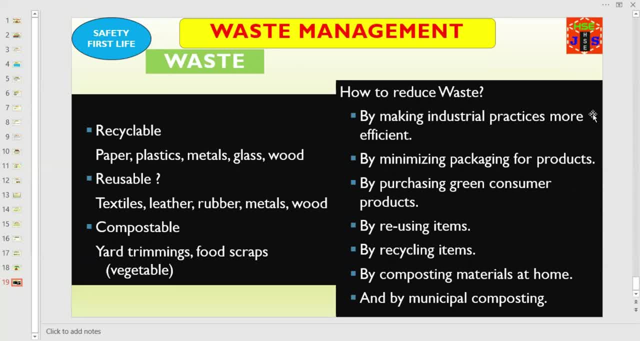 waste. Do you know how we can reduce or minimize waste? By making industrial practices more more efficient, by minimizing packaging for products, by purchasing green consumer products, by reusing items like textiles, leather, rubber, metals or wood. by recycling items. 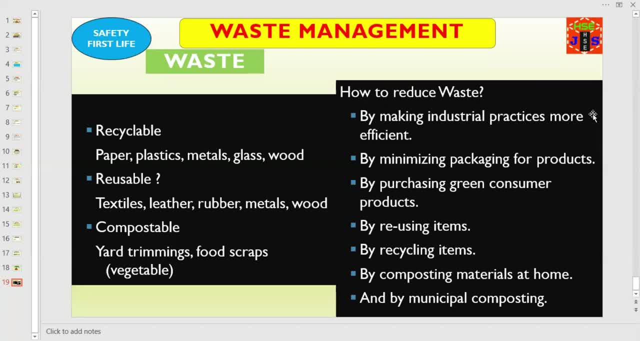 Do you know what are recyclables? Paper, plastics, metals, glass, woods? and by composting materials at home and by municipal composting yard trimmings, food scraps, etc. Just for your kind information Alone, United Arab Emirates is losing 3.5 billion.